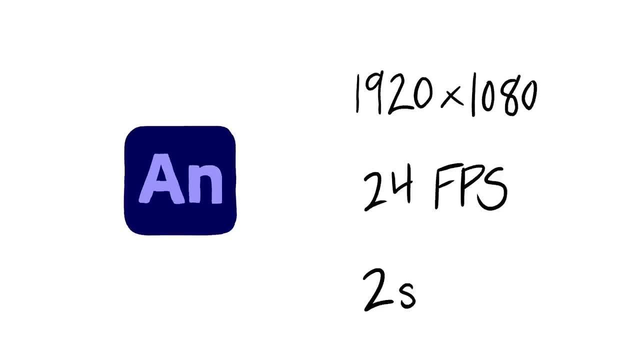 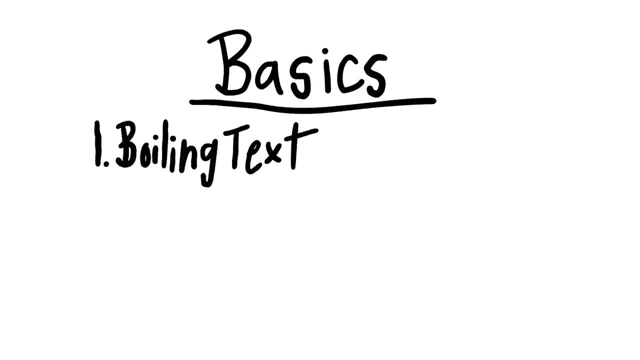 means how many frames are shown in a second, and I'll be animating on twos, which basically means I'll be drawing one out of every two frames, cutting our work in half. This is my first time doing any sort of animation, so we have to start with the basics. Number one boiling text: Write. 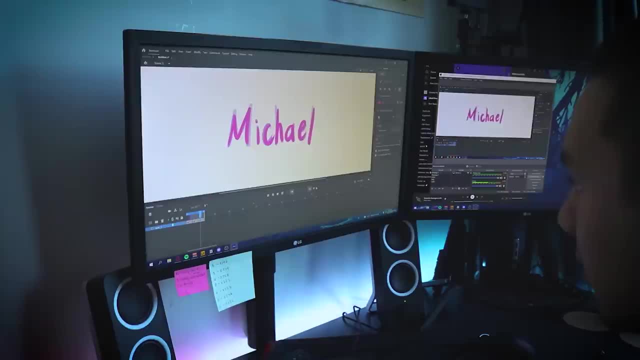 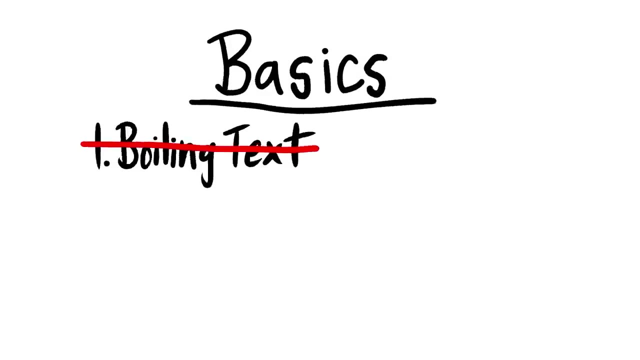 some text three times on three keyframes. Number two: bouncing ball. When animating a bouncing ball, you have to keep these principles in mind: Timing and squash and stretch. The ball accelerates as it falls, which means you have to space your frames further apart as it falls towards the ground. vice versa. 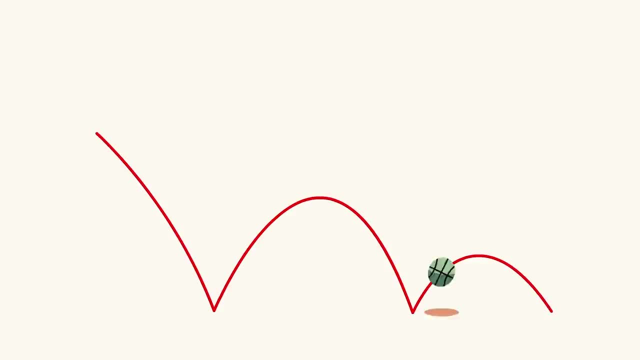 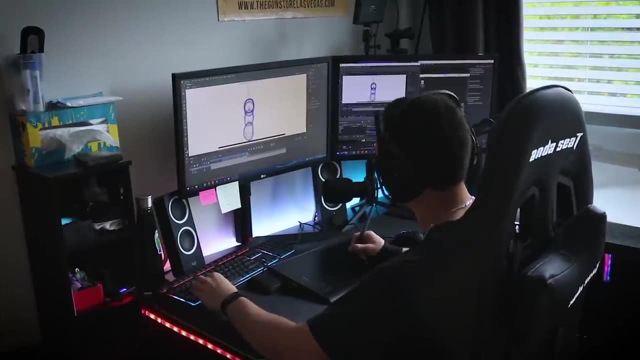 as the ball bounces up and gradually loses momentum for every next bounce until coming to a stop, You can change the amount of squash and stretch to show how light or heavy the ball is. After 20 minutes and 52 frames drawn later, this is my result. 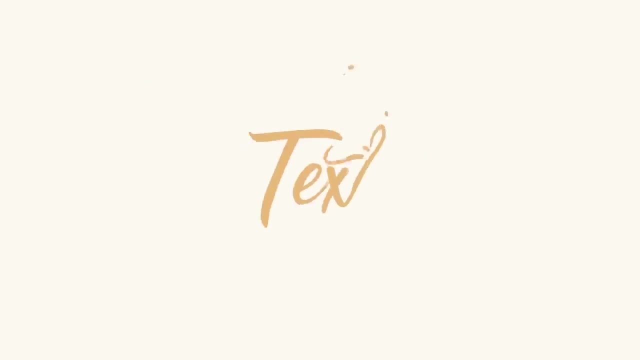 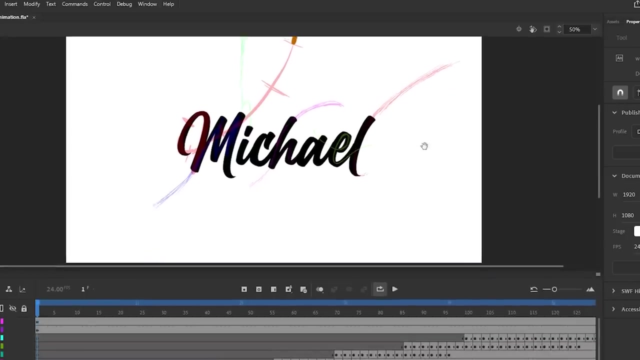 Number three: liquid text. This is a very tedious yet satisfying process. You want to make the full text present, so you have an outline to follow. Now make guides for the liquid animation to follow arcs and use easing to change the tempo. Add little splashes for details. 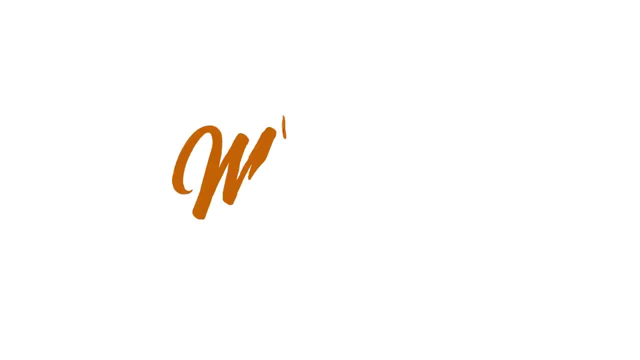 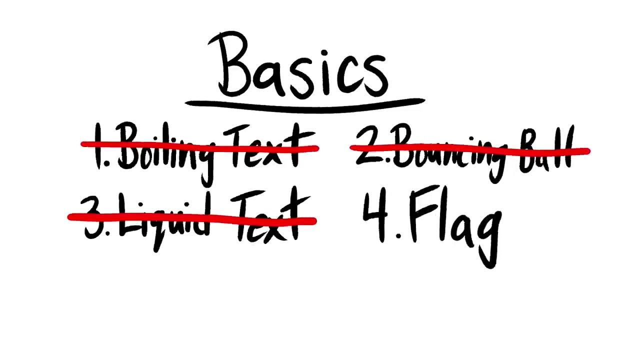 170 frames later and you'll get something like this. I'm super happy with this one. Number four flag animation. Draw each frame of the flag, imagining the wind morphing the flag into the next shape. Duplicate your line and connect them to complete the shape. 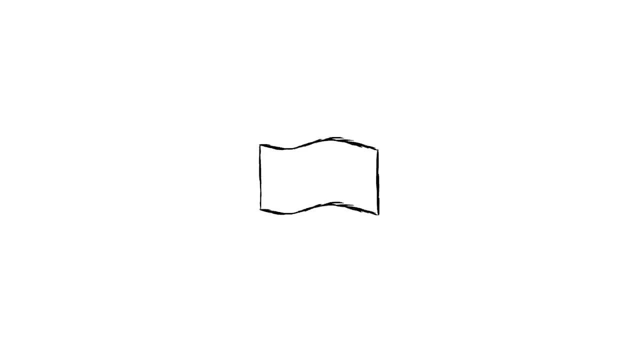 You can use less frames to make the wind stronger And you'll end up with something like this. Number five: the walk cycle. There are endless possibilities when it comes to the walk cycle and it seems super overwhelming. Stick with me. The main poses in a walk cycle is the contact and passing. 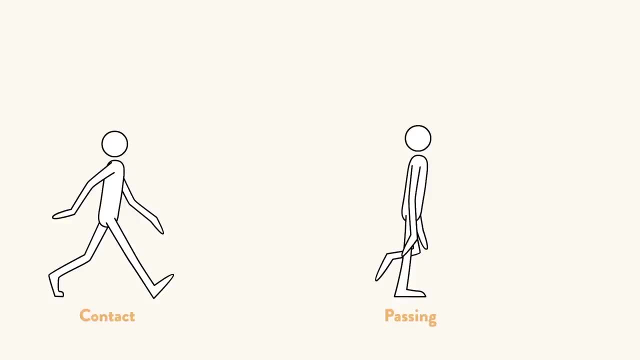 This will already look plausible, but will look very flat. to make it more fluid, We add two more poses called the up and down pose. This will result in your walk cycle being more fluid because we are mimicking the bobbing that happens naturally while walking. 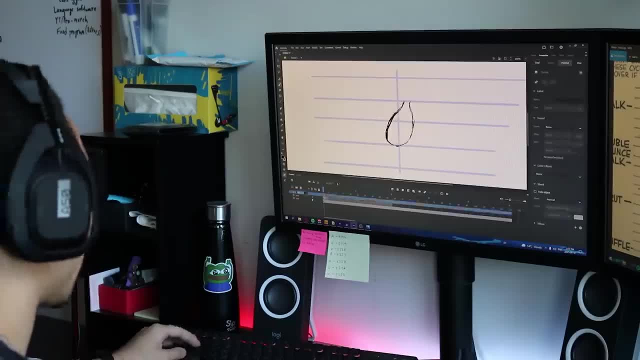 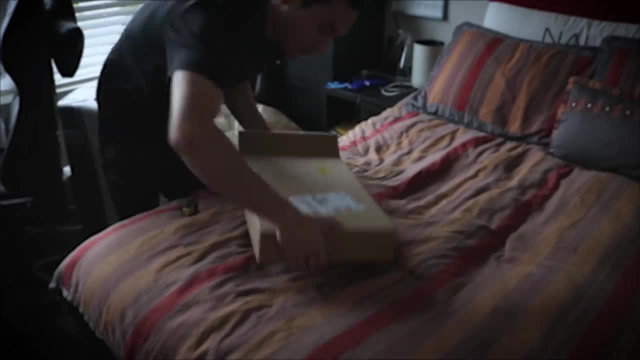 Adding in between frames will make it even smoother. One hour and 30 minutes later, this is my result. Yo Michael from the future here. It's actually been several days since I started making this video and I already upgraded my animation setup.